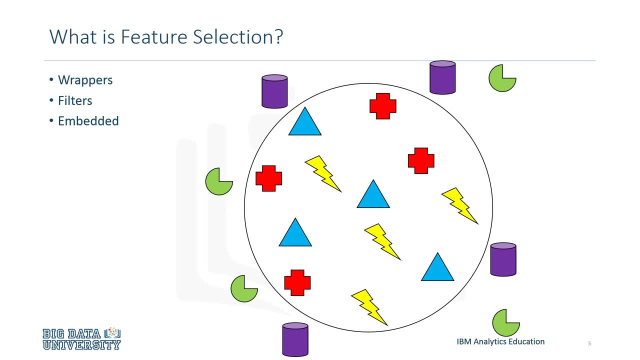 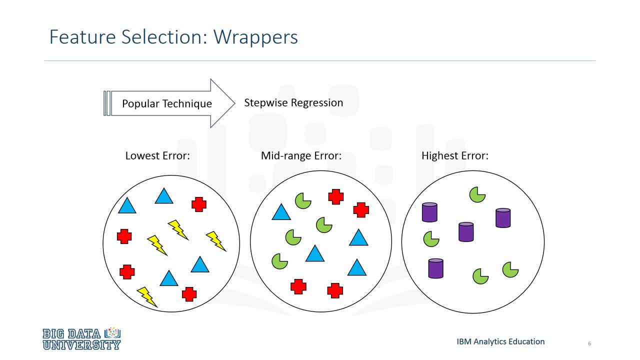 we reduce the amount of strain on the system and produce better results. Wrappers use a predictive model that scores feature subsets based on the error rate of the model. While they're computationally intensive, they usually produce the best selection of features. A popular technique is called Stepwise Regression. It's an algorithm that adds the best feature. 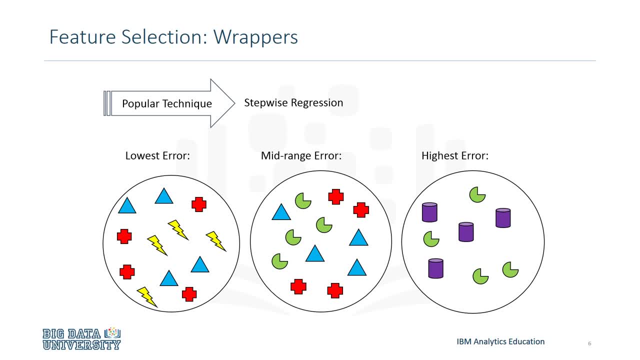 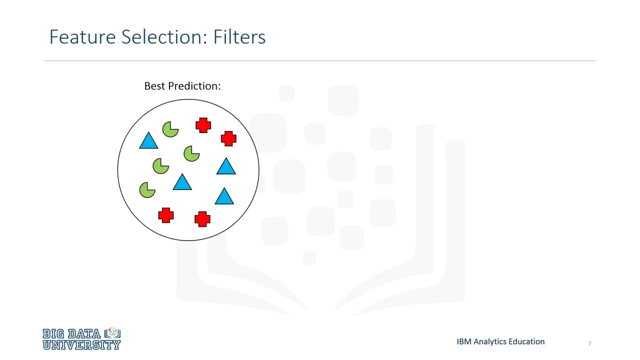 or deletes the worst feature at each iteration. Filters use a proxy measure which is less computationally intensive but slightly less accurate. So it might have a good prediction, but it still may not be the best. Filters do capture the practicality of the data set, but in comparison to error measurement. 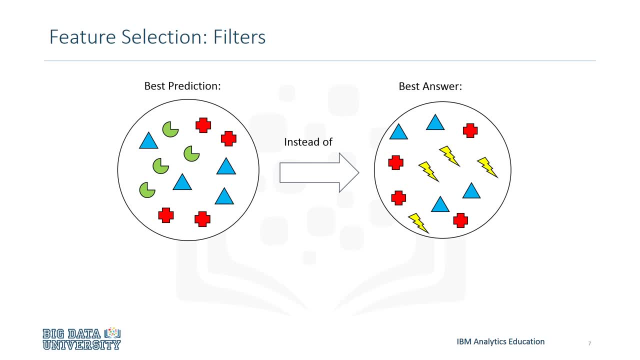 the feature set that's selected will be more general than if a wrapper was used. An interesting fact about filters is that the data set that's selected will be more general than if a wrapper was used. An interesting fact about filters is that the data set that's selected will be more general than if a wrapper was used. 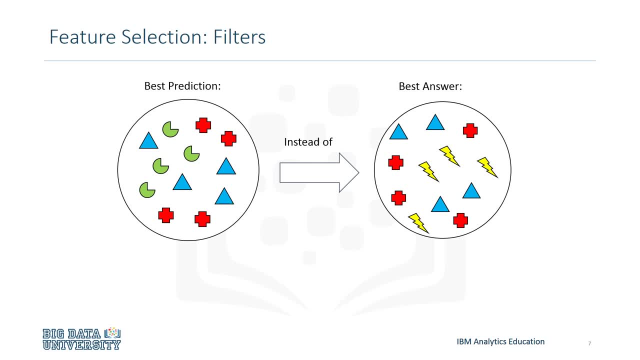 Filters' most common type is that they produce a feature set that don't contain assumptions based on the predictive model, making it a useful tool for exposing relationships between features, such as which variables are bad together and, as a result, drop accuracy, or good together and therefore raise the accuracy. 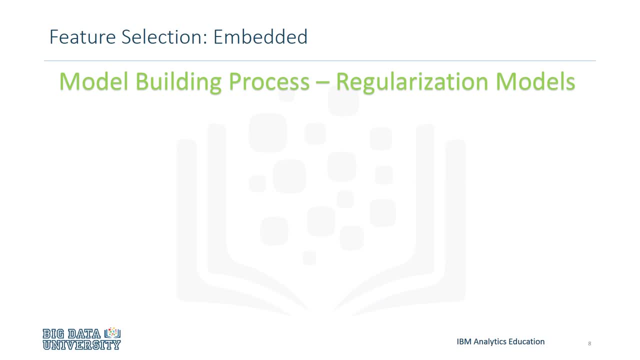 Embedded algorithms learn about which features best contribute to an accurate model during the model-building process. The most common type is called a regular algorithm. The access Twitter account is for Campaigns web search model. In our shape example it would be similar to picking the shapes, or good. 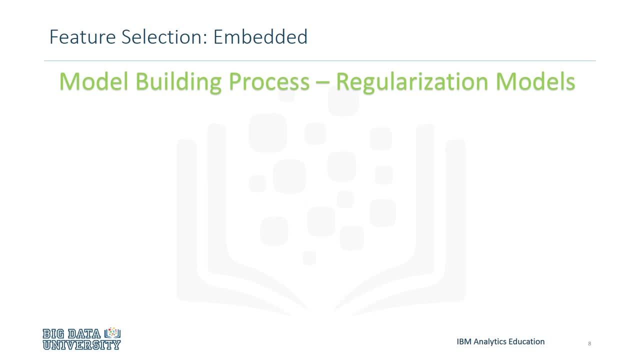 features in each step of the model building process. It might be picking the triangle feature in step 1,, picking the cross feature in step 2, or picking the lightning feature in step 3 to obtain our accurate model Feature. extraction is the process of transforming or projecting a space composing of many 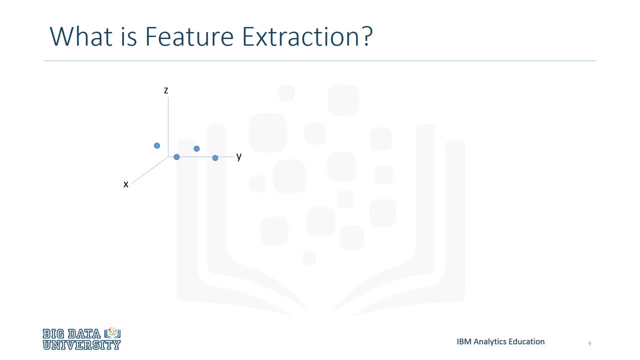 dimensions into a space of fewer dimensions. This is similar to representing data in multiple dimensions to ones that are less. This is useful for when you need to keep your information but want to reduce the resources that it may consume. during processing, The main linear technique is called principal.